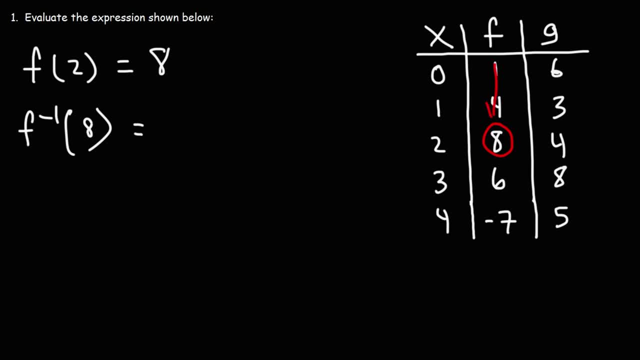 So the inverse of f, of 8, it gives us the x value, which is 2.. It's simply the opposite. So when dealing with inverse functions you need to reverse x and y. So when you're evaluating a function like f, g or h, you're looking for the y value, So the y value corresponds. 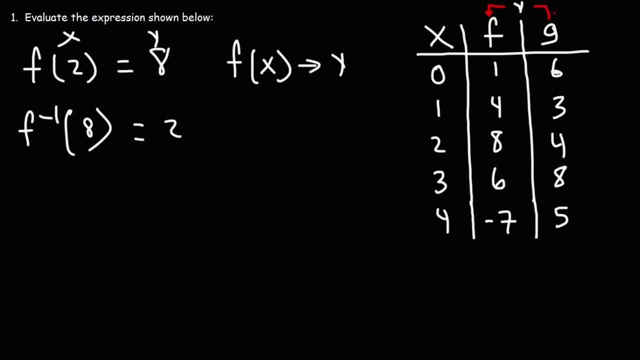 to the last two columns, It's the value of f and g. When you're trying to find the inverse, the number inside is y and it's going to give you x. So if you're trying to evaluate the inverse function, you're looking for the x. 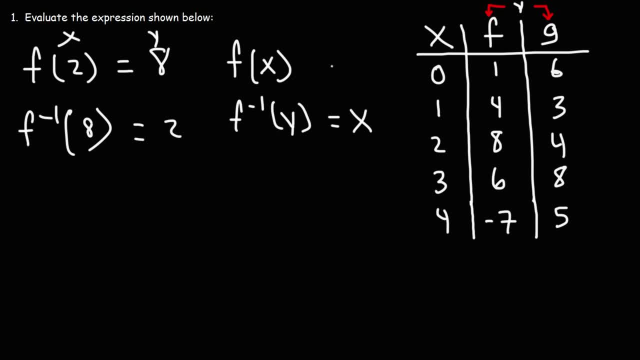 value. If you're trying to evaluate a regular function, you're looking for the y value. So, with that being said, what is the inverse of f of negative 7?? What's the answer to this problem? In other words, f of what number is equal to negative 7?? 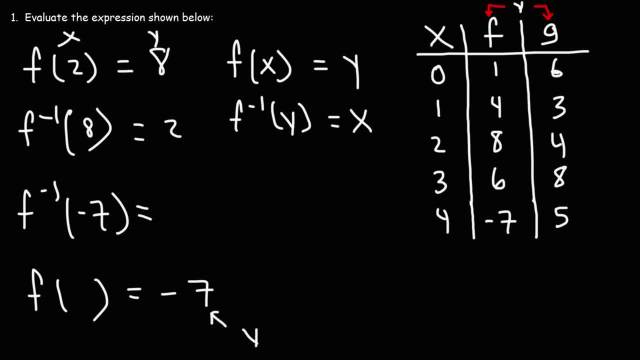 Negative 7 is the y value. What we're trying to find is the x value. So let's look at f and let's see where it's equal to negative 7.. So f is equal to negative 7. here, The answer we're looking for is the x value, So it's 4.. 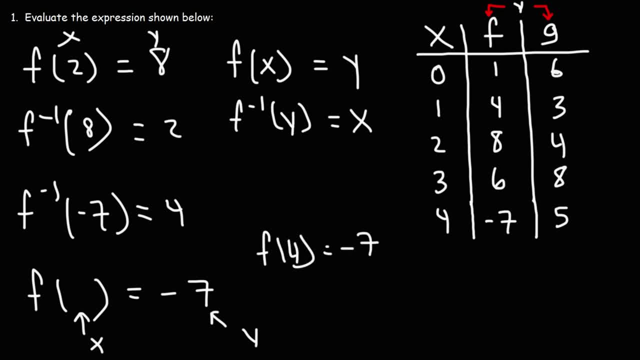 f of 4 is negative 7.. So the inverse of f of negative 7 is 4.. Go ahead and try these problems. Find the value of g of 0,, f of 2, g of the inverse of g of 5,. 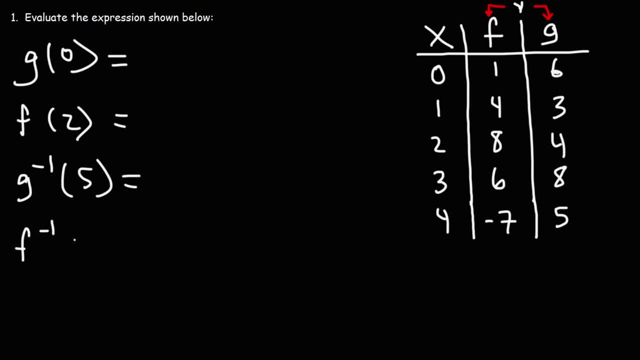 and the inverse of f of 1.. So g of 0, we're looking at g. x is 0.. The y value is 6.. f of 2, x is 2.. We're looking at f. This corresponds to f of 1.. 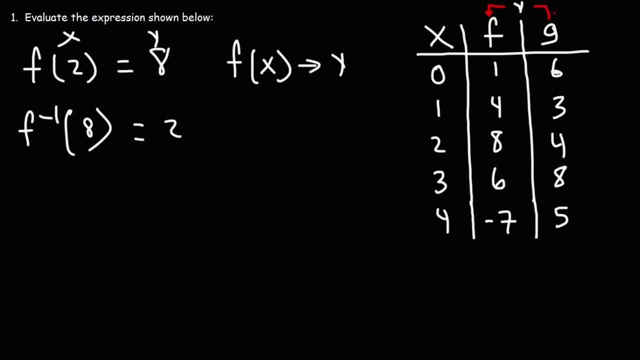 to the last two columns, It's the value of f and g. When you're trying to find the inverse, the number inside is y and it's going to give you x. So if you're trying to evaluate the inverse function, you're looking for the x. 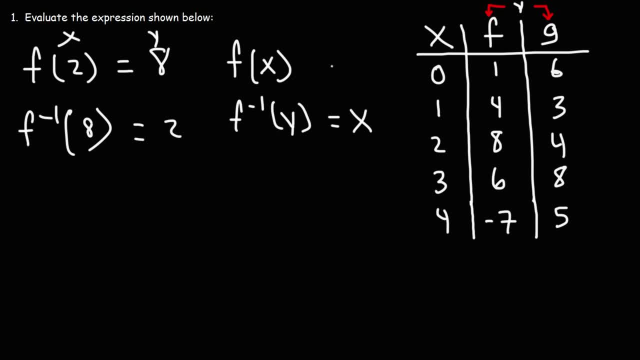 value. If you're trying to evaluate a regular function, you're looking for the y value. So, with that being said, what is the inverse of f of negative 7?? What's the answer to this problem? In other words, f of what number is equal to negative 7?? 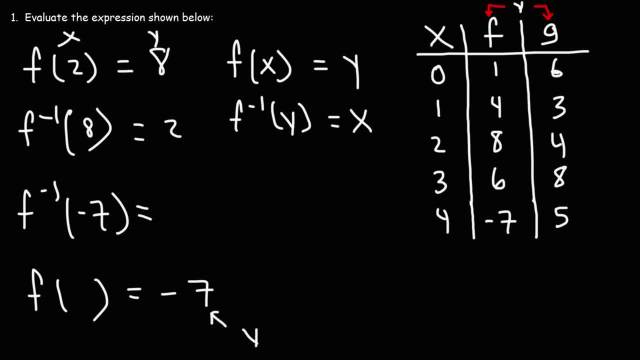 Negative 7 is the y value. What we're trying to find is the x value. So let's look at f and let's see where it's equal to negative 7.. So f is equal to negative 7. here, The answer we're looking for is the x value, So it's 4.. 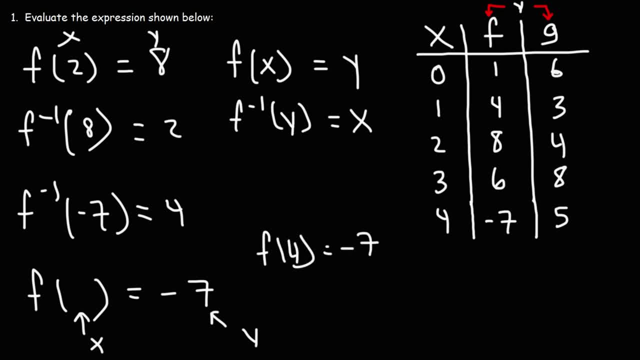 f of 4 is negative 7.. So the inverse of f of negative 7 is 4.. Go ahead and try these problems. Find the value of g of 0,, f of 2, g of the inverse of g of 5,. 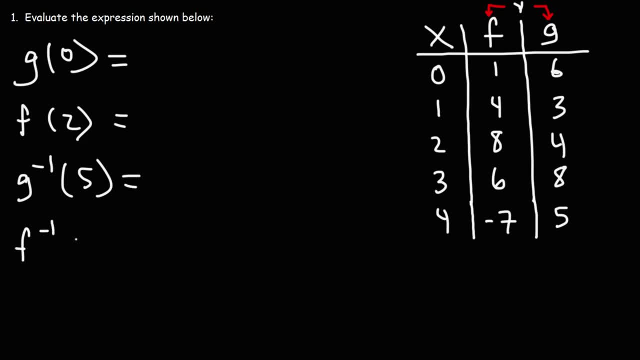 and the inverse of f of 1.. So g of 0, we're looking at g. x is 0, the y value is 6.. f of 2, x is 2, we're looking at f. f of 2, x is 2, we're looking at f. 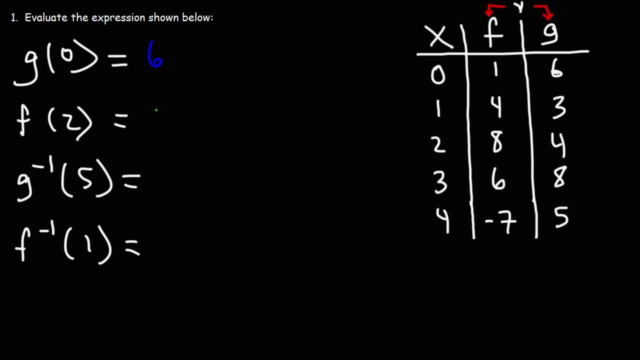 corresponds to a y value of 8. The inverse of g of 5.. So we're dealing with g Now. the 5 is not an x value, it's a y value. We're looking for the x value. The x value that corresponds to that is 4.. 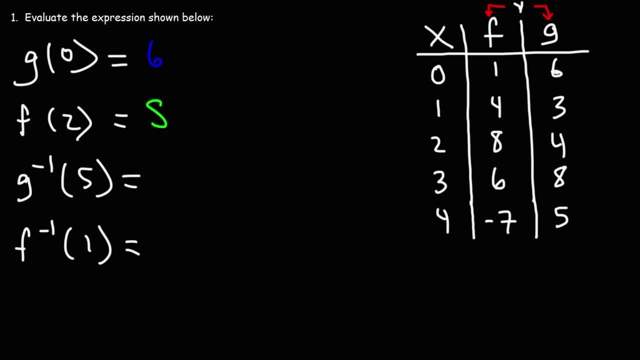 to a y value of 8. The inverse of g of 5.. So we're dealing with g Now. the 5 is not an x value, it's a y value. We're looking for the x value. The x value that corresponds to that is 4.. 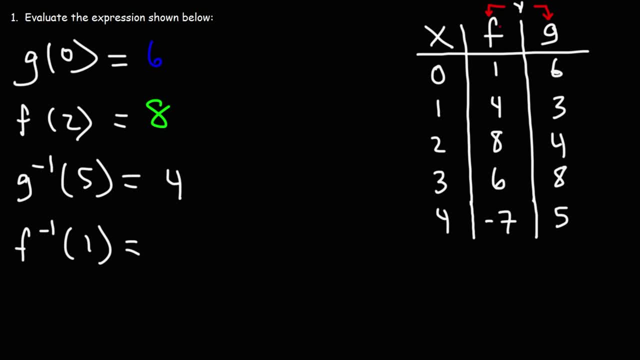 Now what about the inverse of f of 1?? So we're looking at f, the y value is 1, the corresponding x value is 0. So remember this when you're evaluating regular functions like these two: this should be a 0.. I don't know why I put an x here. 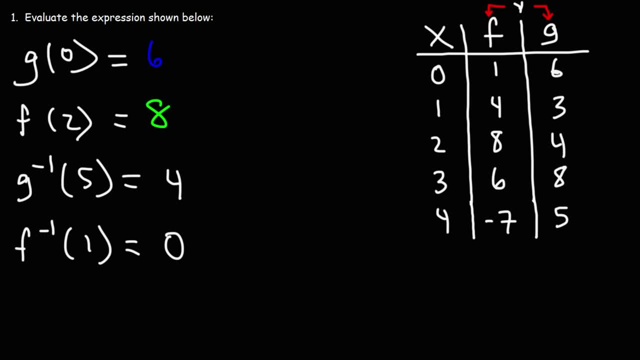 That's what happens when you get old. So whenever you're evaluating the regular functions, you're looking for the y value. When you're evaluating the inverse functions, you're looking for the x value. So the inverse of f of 1 is 0.. The inverse of g of 5 is 4.. 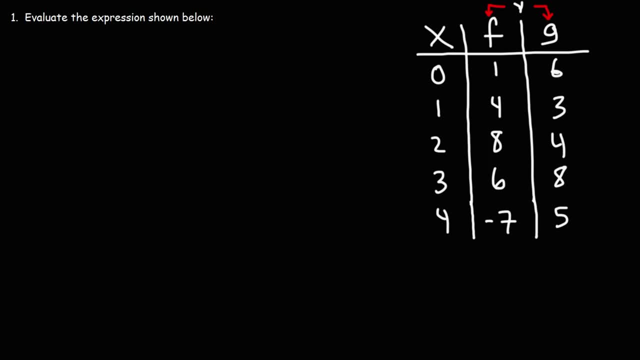 So now that we know how to do that, let's work on some harder problems. Try these two problems. Let's move on to composite functions. Find the value of f of 1.. Find the value of f of g of 1, and also the inverse of f of g of 2.. 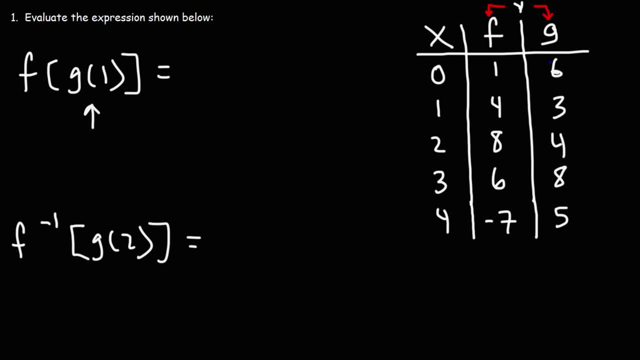 So let's work on the inside g of 1. We're looking for the y value. Here's g, here's 1. The y value is 3.. So now we're looking for f of 3.. So we're looking for another y value: Here's f, here's 3.. 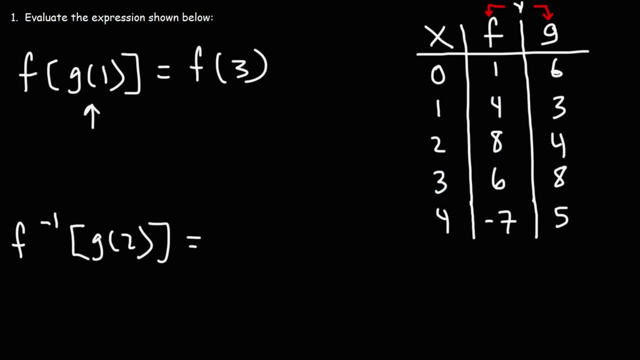 The y value is 6.. So f of g of 1 is 6.. Now let's move on to the next one. What is g of 2?? So we have: g of 2 is 4.. So now we have the inverse of f of 4.. 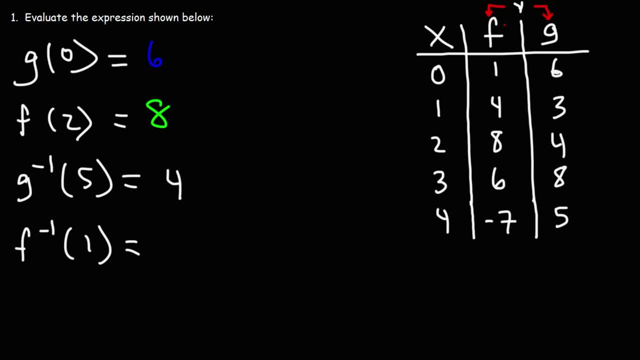 Now what about the inverse of f of 1?? So we're looking at f, the y value is 1, the corresponding x value is 0. So remember this when you're evaluating regular functions like these two: this should be a 0.. I don't know why I put an x here. 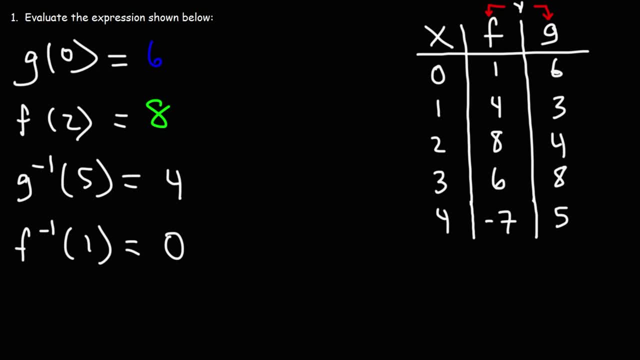 That's what happens when you get old. So whenever you're evaluating the regular functions, you're looking for the y value. When you're evaluating the inverse functions, you're looking for the x value. So the inverse of f of 1 is 0.. The inverse of g of 5 is 4.. 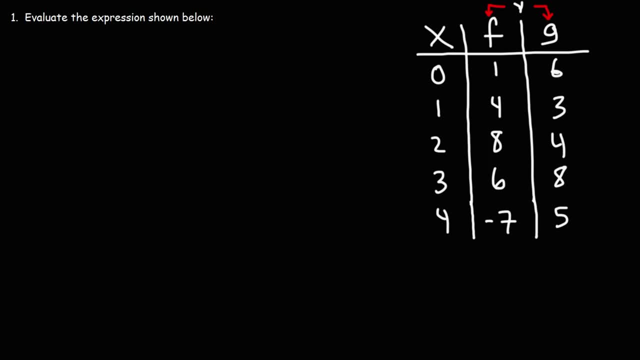 So now that we know how to do that, let's work on some harder problems. Try these two problems. Let's move on to composite functions. Find the value of f of 1.. Find the value of f of g of 1, and also the inverse of f of g of 2.. 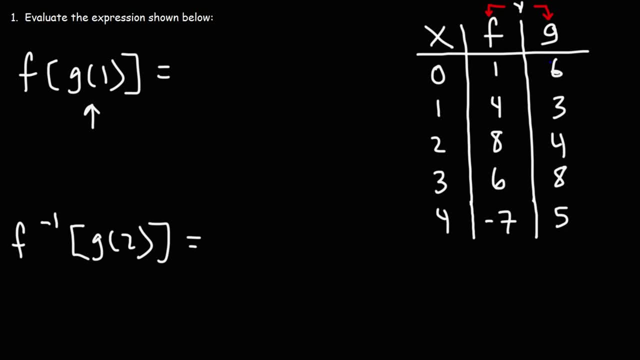 So let's work on the inside g of 1. We're looking for the y value. Here's g, here's 1. The y value is 3.. So now we're looking for f of 3.. So we're looking for another y value: Here's f, here's 3.. The y value is 6.. 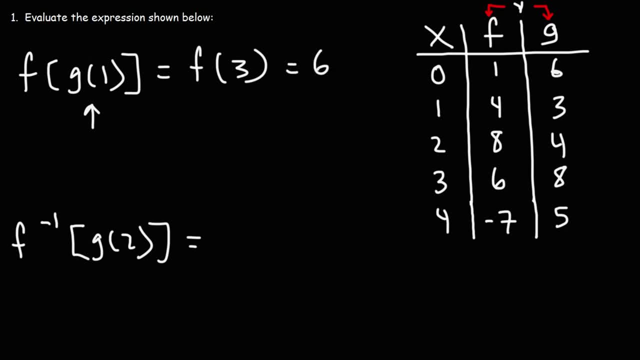 So f of g of 1 is 6.. Now let's move on to the next one. What is g of 2?? So we have: g of 2 is 4.. So now we have the inverse of f of 4.. 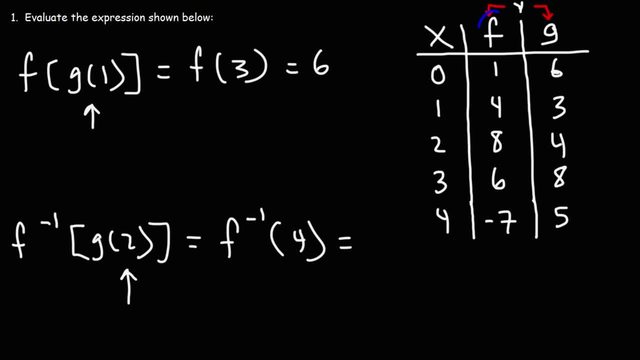 So we're looking for an x value Starting with f. the y value is 4.. The corresponding x value is 1.. So the inverse of f of 4 is 1.. Go ahead and try these two problems. First f. 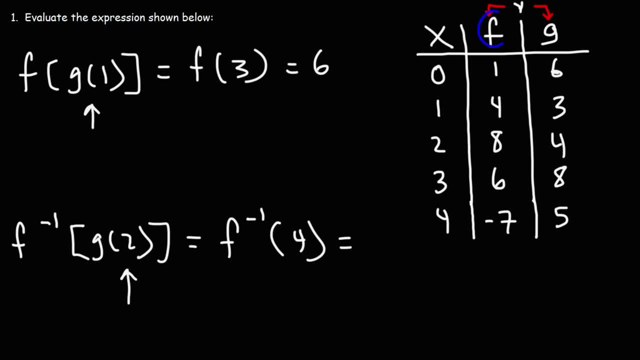 So we're looking for an x value Starting with f. the y value is 4.. The corresponding x value is 1.. So the inverse of f of 4 is 1.. Go ahead and try these two problems. First, f inverse of g. 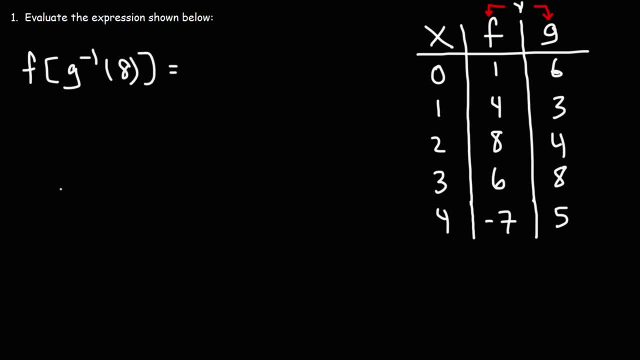 f inverse of g of 8, and also the inverse of g and the inverse of f of negative 7.. So go ahead and work on those two problems. So let's start with this: What is the inverse of g of 8?? 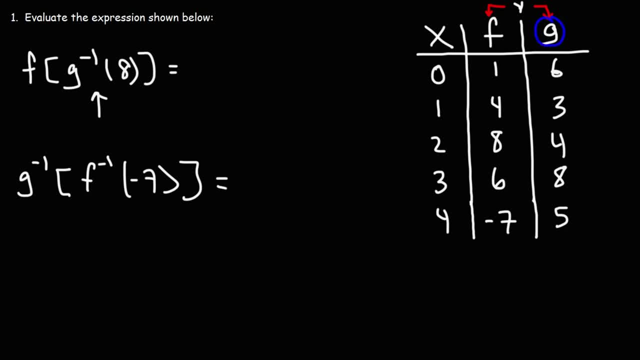 What is the inverse of g of 8?? So we have g, We're going to find where it's equal to 8, and that's here, And we're looking for the x value. So that is 3.. So now we have. 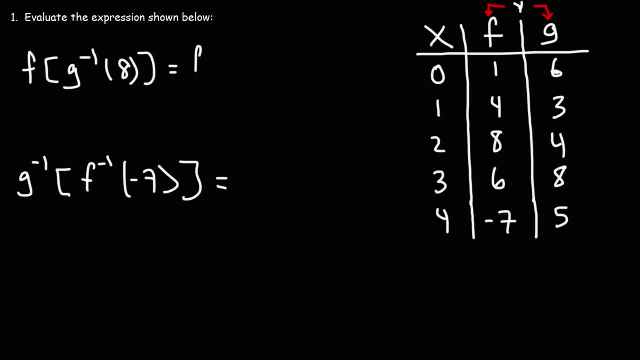 f of 3.. So now let's evaluate f of 3.. So we got: f of 3 is 6.. So that's it for that problem. For the next one, we have the inverse of f of negative 7.. So here's negative 7 in the f column. 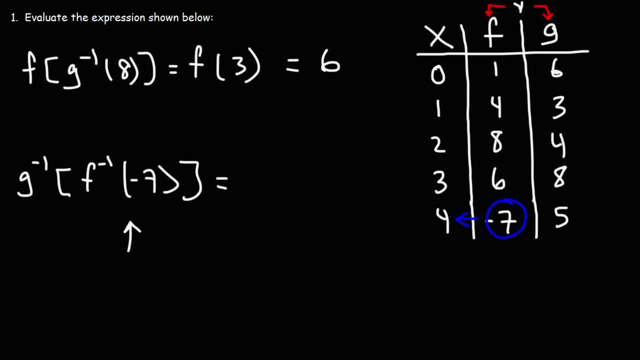 The x value that corresponds to that is 4.. So now we're looking for the inverse g of 4.. So, looking at column g, here's the 4.. The x value is 4.. The x value that corresponds to that is 2.. 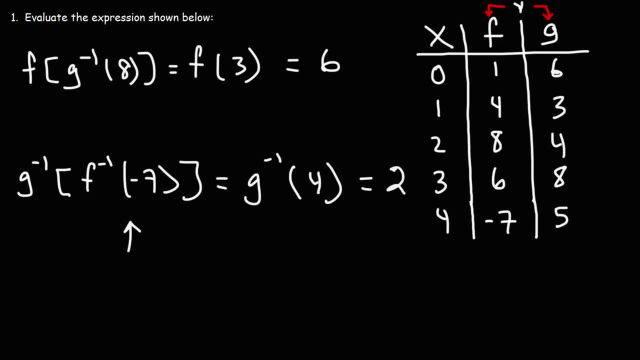 So that's it for the second example. Once you do this after a while, it gets easier. So now that you're getting the hang of this, let's try some harder problems. Try these two: The inverse of f and the inverse of g of 3.. 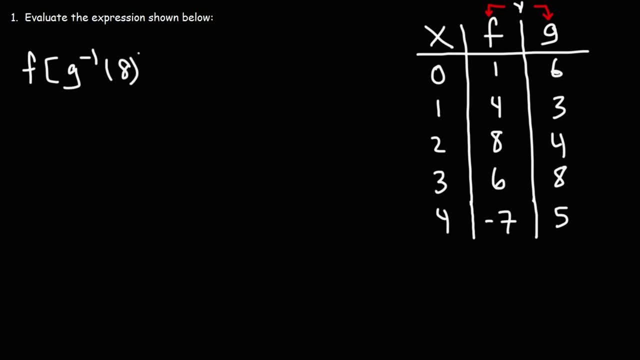 Inverse of g of 8. And also the inverse of g and the inverse of f of negative 7.. So go ahead and work on those two problems. So let's start with this: What is the inverse Inverse of g of 8.. 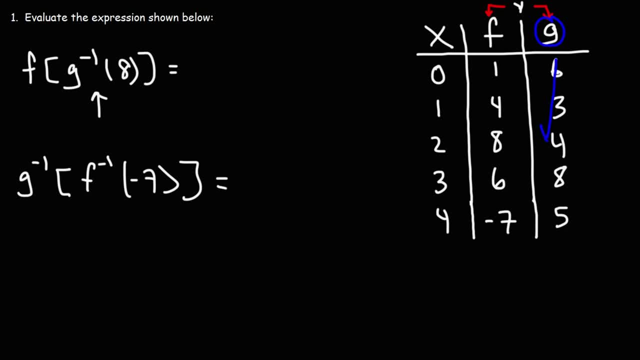 So we have g, We're going to find where it's equal to 8, and that's here. And we're looking for the x value. So that is 3.. So now we have f of 3.. So now let's evaluate f of 3.. 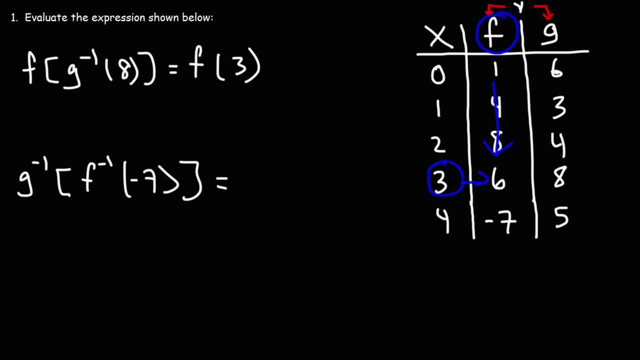 So we got f of 3.. f of 3 is 6.. So we're going to have f of 3.. So the x value is 6.. So that's it for that problem. For the next one, we have the inverse of f of negative 7.. 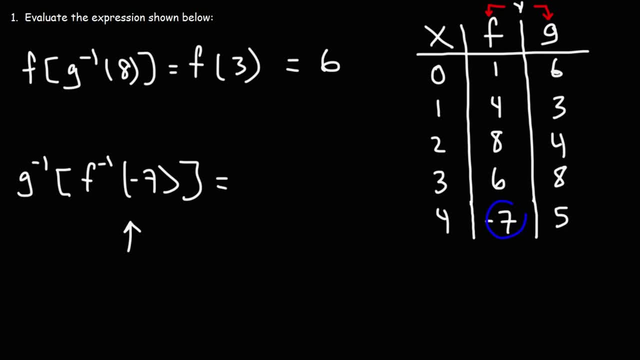 So here's negative 7 in the f column. The x value that corresponds to that is 4.. So now we're looking for the inverse g of 4.. So looking at column g, Column G, here's the 4, the x-value that corresponds to that is 2.. 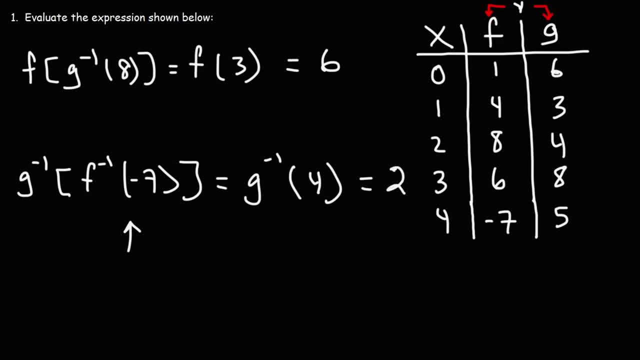 So that's it for the second example. Once you do this after a while, it gets easier. So now that you're getting the hang of this, let's try some harder problems. Try these two: Find the inverse of f and the inverse of g of 3.. 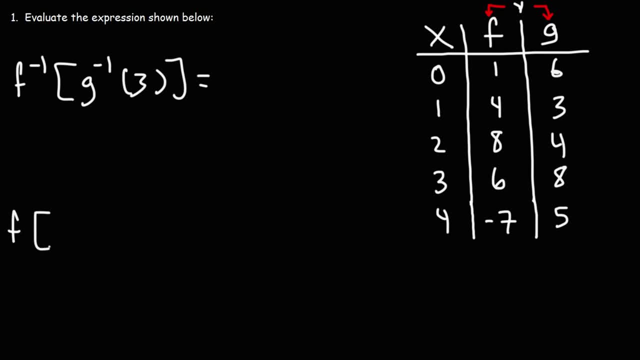 For the next one, we're going to have three functions: f of g, of the inverse of f of 4.. Go ahead and try those two problems. So let's start with this: The inverse of g of 3.. So, looking at the g-column, 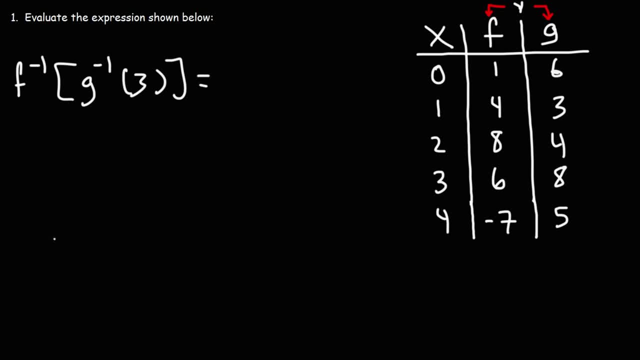 So let's try this. For the next one, we're going to have three functions: f of g, of the inverse of f of 4.. Go ahead and try those two problems. So let's start with this: The inverse of g of 3.. 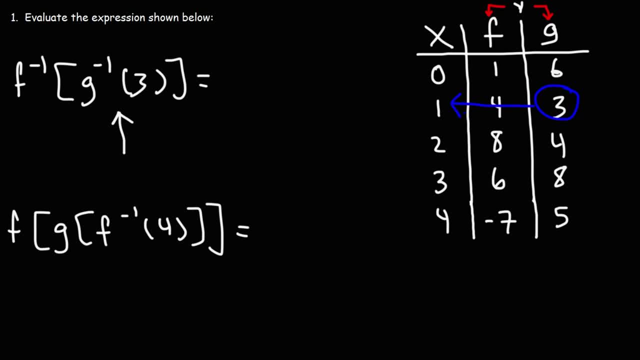 So, looking at the g column, we find 3, and then find the corresponding x value, which is 1.. So now we have the inverse of f, of 3.. So now let's look at the f column, Find 1, and find the corresponding x value, which is 0. 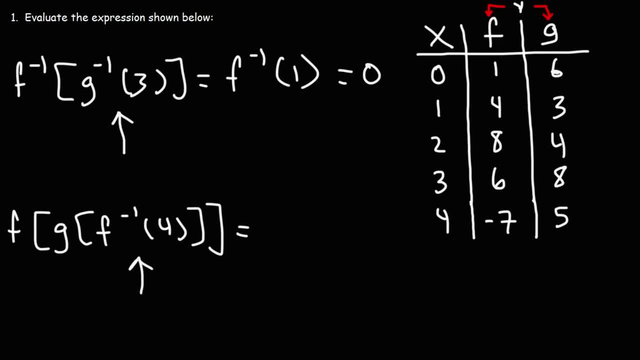 Moving on to the next one, The inverse of f of 4.. So, focusing on the f column, here's 4.. The corresponding x value is 1.. So f of the inverse of f of 4 is 1.. So now we have f of g of 3.. 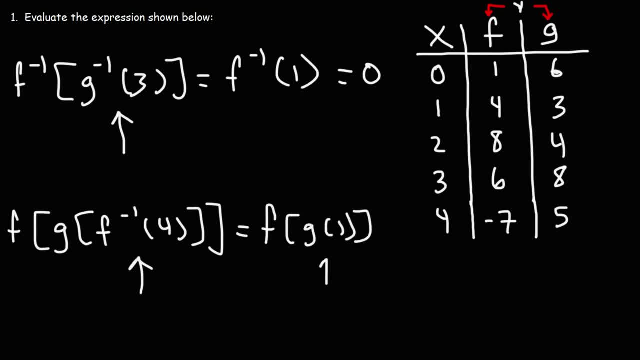 So now we have f of g of 3. So now we have f of g of 3. So now we have f of g of 1. So now we can evaluate g of 1.. So x is 1 and we get 3.. 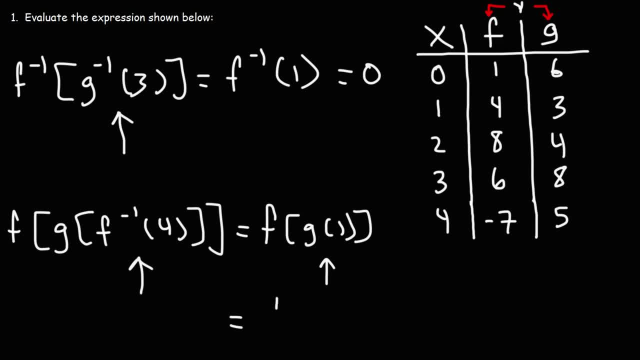 So g of 1 is 3.. We're looking for the y value this time. So now we have f of 3.. So x is 3.. We're looking at the f column, that corresponds to 6.. So that's it for that one. 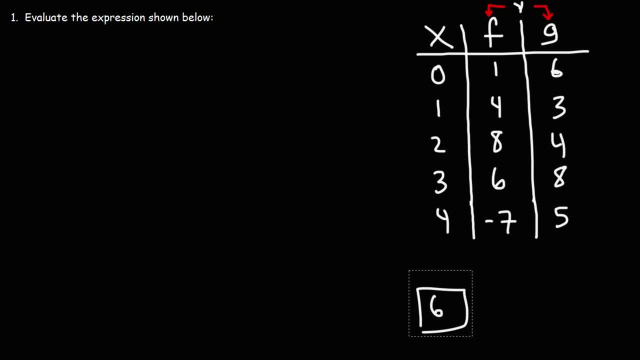 Now, for the sake of practice, let's work on one more example. Let's say we have the inverse of f and then of g, and then another inverse of f of 6.. Go ahead and try that. So the inverse of f of 6.. 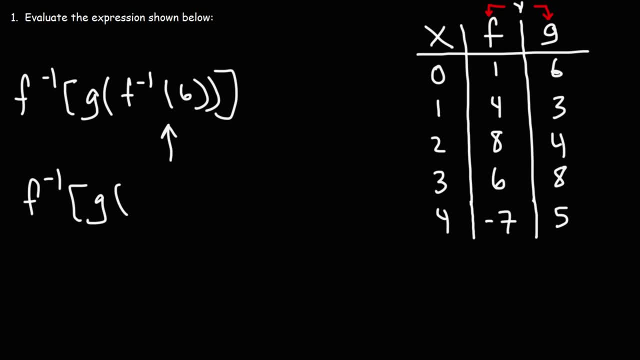 Let's start with that, So the inverse of f of 6.. Let's start with that, So the inverse of f of 6.. So, looking at the f column, let's find the y value of 6, and then the corresponding x. 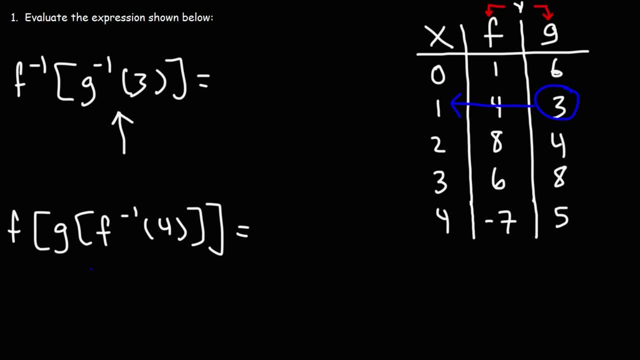 We find 3, and then find the corresponding x-value, which is 1.. So now we have the inverse of f of 1.. So now let's look at the f-column, Find 1, and find the corresponding x-value, which is 0.. 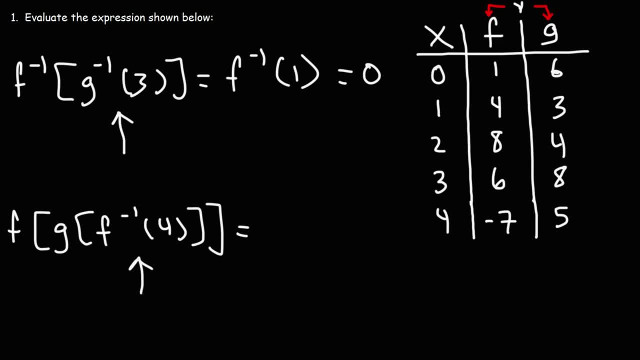 Moving on to the next one, The inverse of f of 4.. So, focusing on the f-column, here's 4.. The corresponding x-value, The corresponding x-value is 1.. So the inverse of f of 4 is 1.. 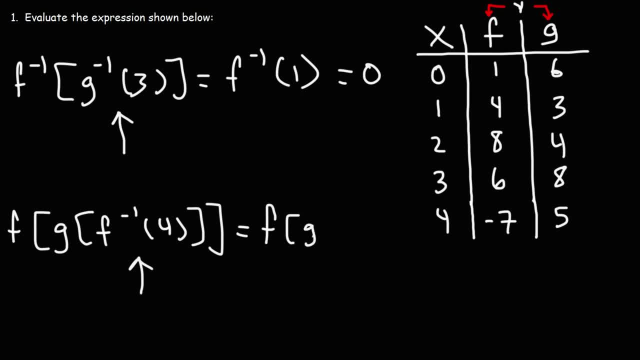 So now we have f of g of 1.. So now we can evaluate g of 1.. So x is 1, and we get 3.. So g of 1 is 3.. We're looking for the y-value this time. 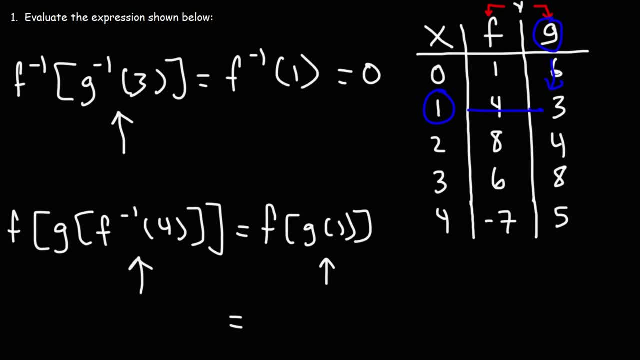 So now we have f of 3. So x is 3.. We're looking at the f-column. That corresponds to 6.. So now we have f of 3. So x is 3.. We're looking at the f-column. 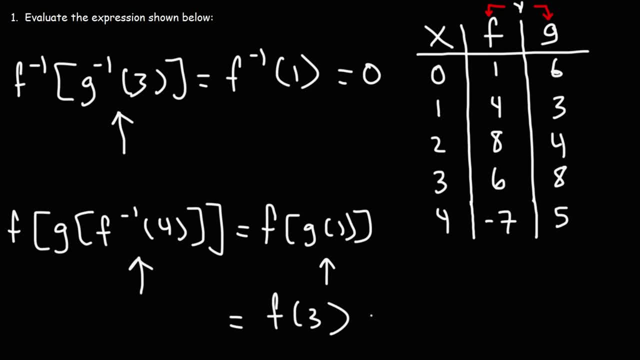 That corresponds to 6.. We're looking at the f-column. So that's it for that one. Now, for the sake of practice, let's work on one more example. Let's say we have the inverse of F and then of g, and then another inverse of f of 6.. 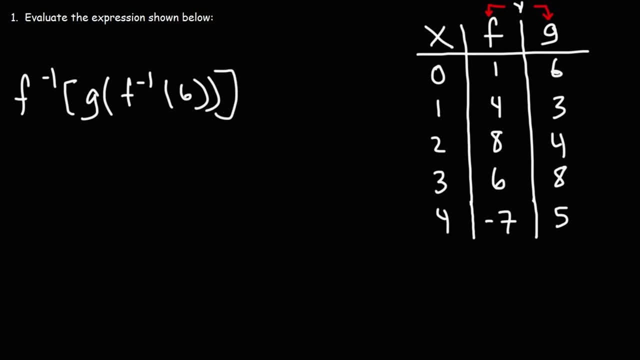 Go ahead and try that. So the inverse of f of 6, let's start with that. So, looking at the f column, let's find the y value of 6, and then the corresponding x value is 3.. So the inverse of f of 6 is 3.. 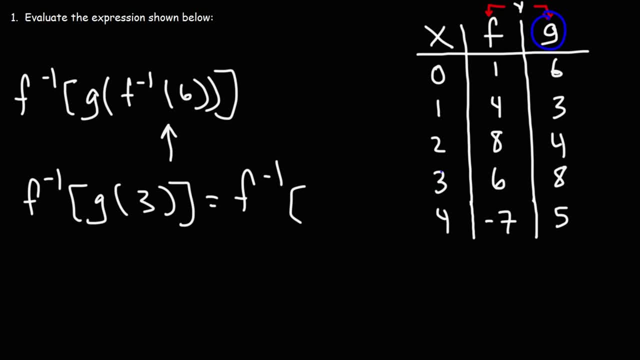 And then g of 3, g of 3 is 8.. Now the inverse of f of 8, so here's f, here's 8, the corresponding x value is 2.. So the final answer for the whole thing is 2..